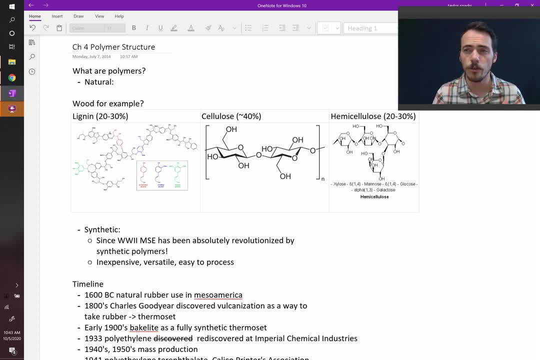 nature, and yet it's a polymeric material. So what's inside of that Wood, for example? Well, 40% of wood is cellulose. right, Cellulose is an interesting polymer. It's a crystalline polymer, meaning it makes up long chains. right, It forms crystals because these long chains can form. 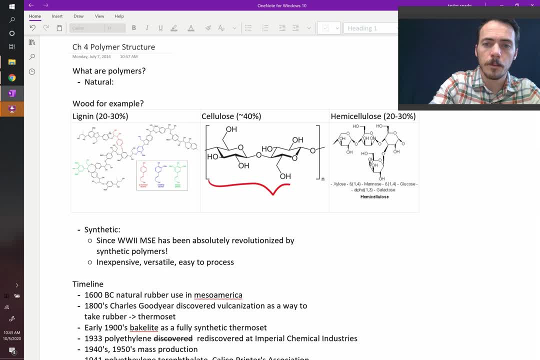 And what are the chains made up of? The chains themselves are made up of these repeat units of that little building block. right, If you put these together like Legos, that's the building block, You can see. it's a ring-like structure. It's got OH groups on the side and 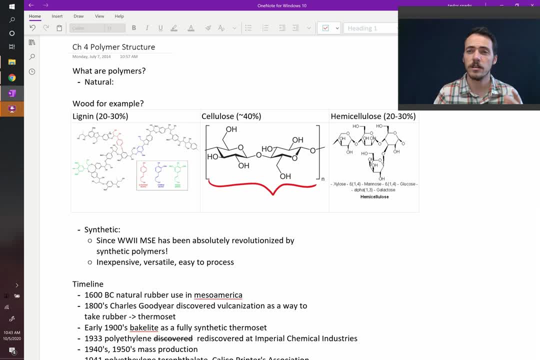 it's got two of them. If you connect enough of those together, you get cellulose right, And that's what a lot of what plants is Cotton shirts are like 100% cellulose- It's almost 100% cellulose cotton shirts right. Also, in wood you've got things like lignin. Look at all these. 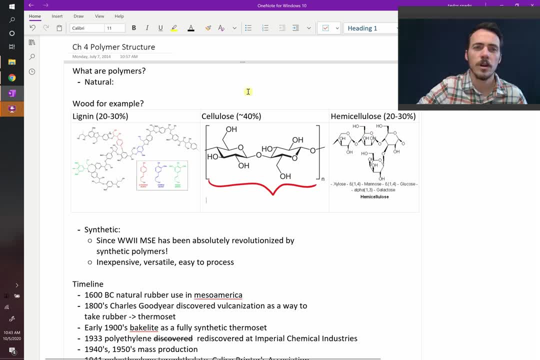 aromatic groups that are on here and it's hemicellulose. So natural polymers very often aren't completely pure right. They exist with many different materials all coming together to make natural polymers. So natural polymers are very often not completely pure right. They exist with. 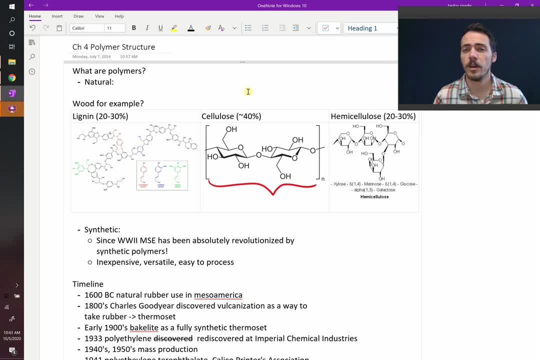 natural polymers. On the other hand, you've got synthetic polymers. Synthetic polymers have only been around for not very long, not very long at all, really. since World War II, which is only a couple of generations back, have we had synthetic polymers, and yet they have completely revolutionized. 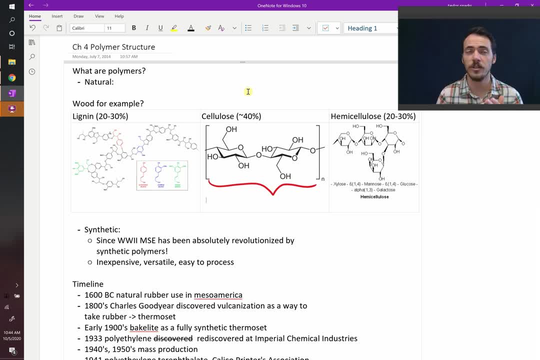 the world. Look around you in your room. By the time you finish this chapter, you'll be able to point to all sorts of polymers that change the way that your life works. because we've made them And why? Why are they such dramatic? 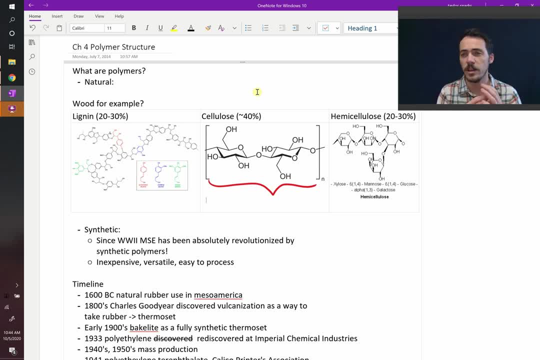 changing materials. They've got awesome properties. They're very easy to process into lots of different shapes, They are inexpensive and they are versatile. You can make them do lots of different things, right? So here's a rough timeline of the polymers that we're going to. 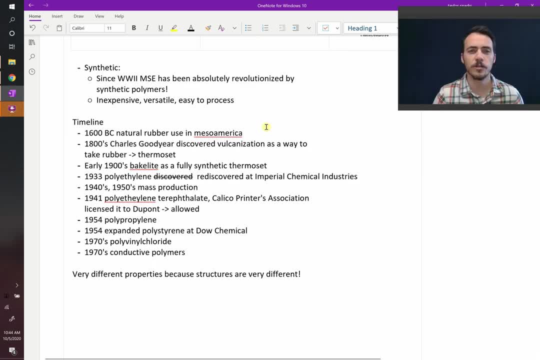 cover in this chapter right Go way back 1600 BC. By the way, if you're interested in more of the history of this particular natural rubber, we did a podcast on it in my material science podcast called Materialism. Check it out if you want. So, 1600 BC: there's evidence that ancient 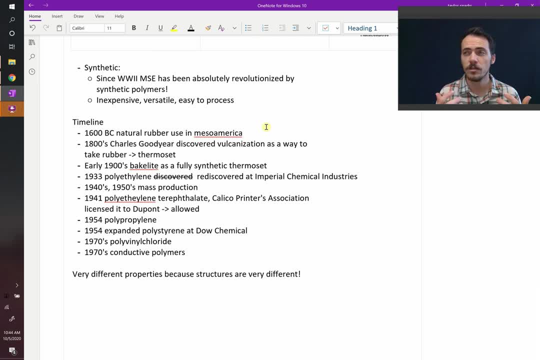 Mesoamericans were using natural rubber from the rubber tree to make things like bouncy balls. right Now, it is not the rubber that we know and love today. We've gotten a lot better at it, And a key part of that process. 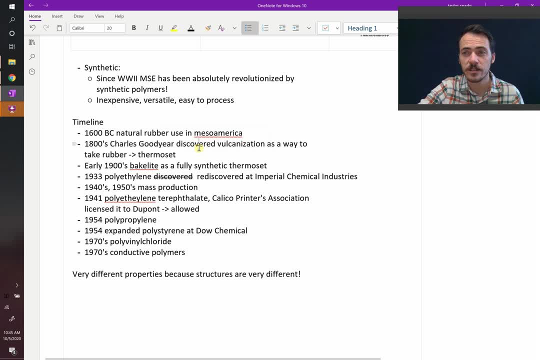 was Charles Goodyear. Like, if you have Goodyear tires, this is the same Goodyear right, Charles Goodyear. he discovered what's called vulcanization- We'll talk more about this this chapter. but it takes a natural rubber and turns it into a thermoset right. That's in the 1800s, So way. 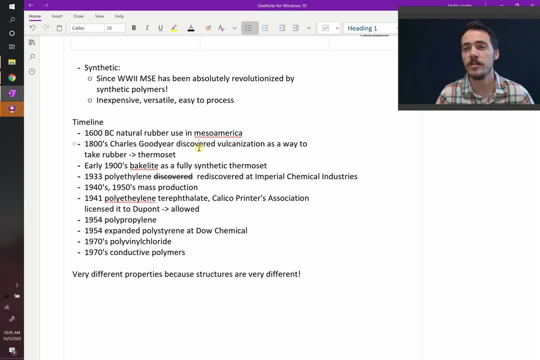 later. Okay, It wasn't until the early 1900s that we discovered Bakelite. This is the fully synthetic thermoset, And we'll talk about what thermoset means soon. And it wasn't until 1933 that polyethylene was discovered. It was not discovered in 1933. It. 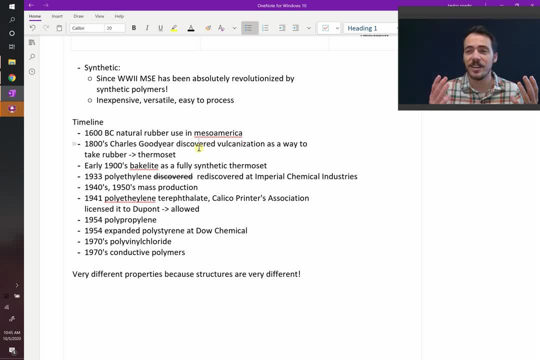 was discovered in 1898 by a couple of Germans, but they didn't know what to do with it And it was hard to make it very useful, And so they accidentally discovered it. And 35 years later it was re-accidentally discovered in imperial chemical industries. And at that point, 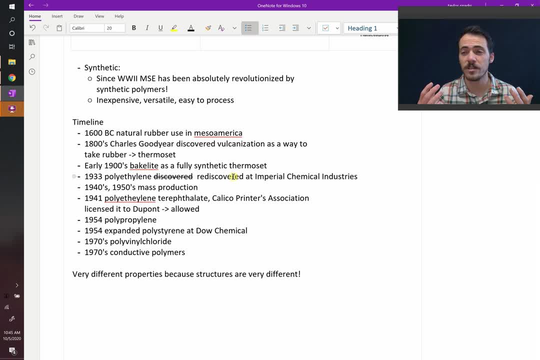 they figured out how to make it reproducibly And really this was the dawn of the synthetic polymer. They realized, holy smokes, this substance is pretty useful And we can. now we know how to make it. We can make all sorts of things out of it, which led to in the World War II era, in 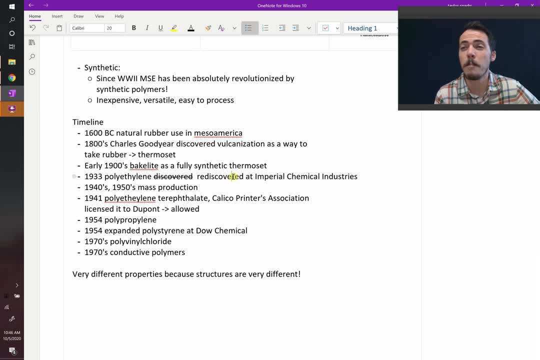 particular as things industrialized 40s and 50s, you started to see mass production of synthetic polymers In the 1941, you get polyethylene terephthalate at Calico Printers Association. This was licensed to DuPont right In 1954, you get polypropylene. Polypropylene is a huge 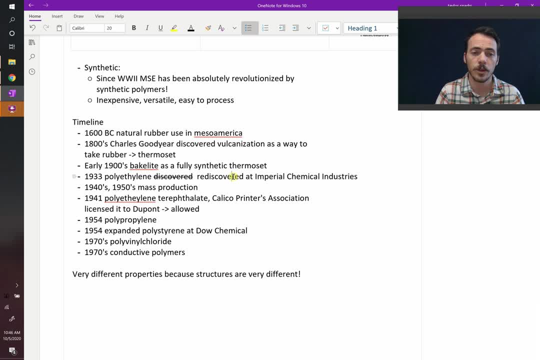 polymer. We use that for lots of stuff In 1954, you get expanded polystyrene. We have another word for that. We call it styrofoam. right, That was Dow Chemical. Styrofoam was incredibly important In the 70s. 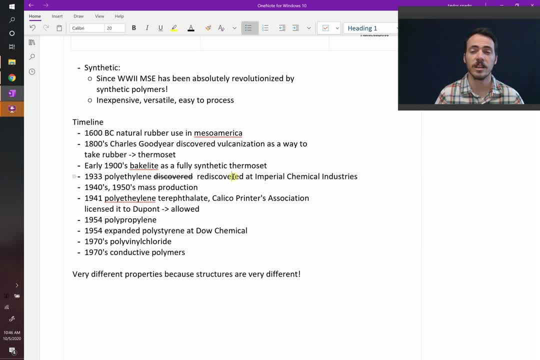 we ended up with polyvinyl chloride And then you started getting conductive polymers And nowadays you know we could go on. They get more and more specialized with more and more cool things that they can do. So, as we've been going through this list, I've said polyethylene, which hopefully 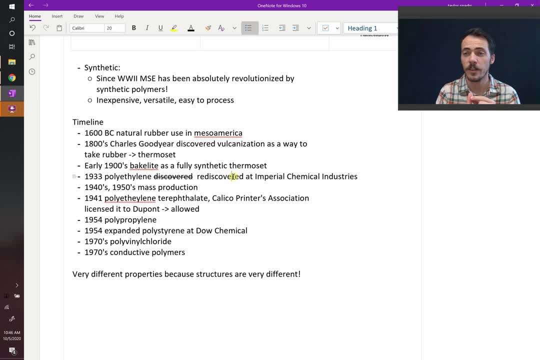 you've seen before HDPE or LDPE. if you've ever seen that, that's polyethylene, We've- we've said bakelite, which is like your grandma's old phone was made out of that from. you know the old days. You've got styrofoam, You've got polypropylene. Hopefully, what you're realizing-